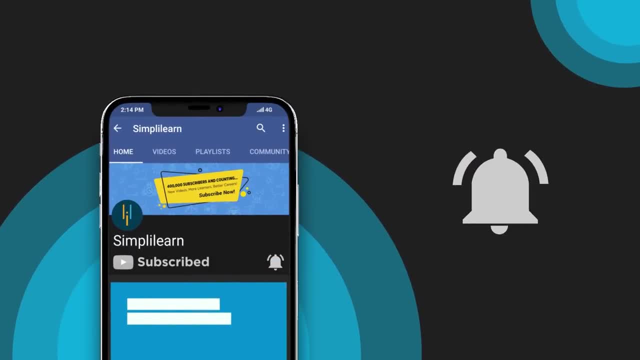 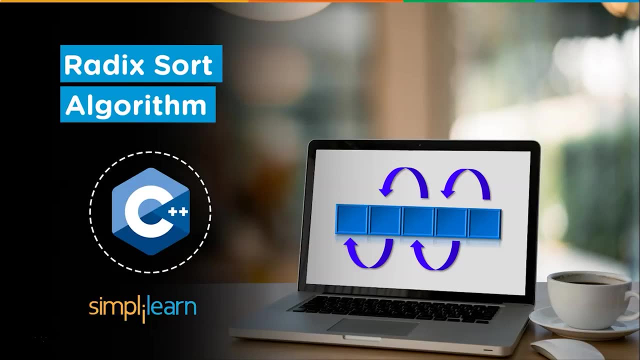 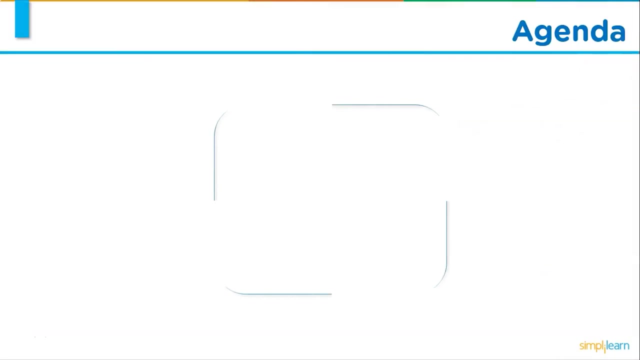 Hey everyone, I am Babakhandelwal and I welcome you all to Simply Learn's YouTube channel. In this session, we will discuss Radix Sort Algorithm. We shall begin our session by introducing Radix Sort. Then we will discuss Radix Sort. 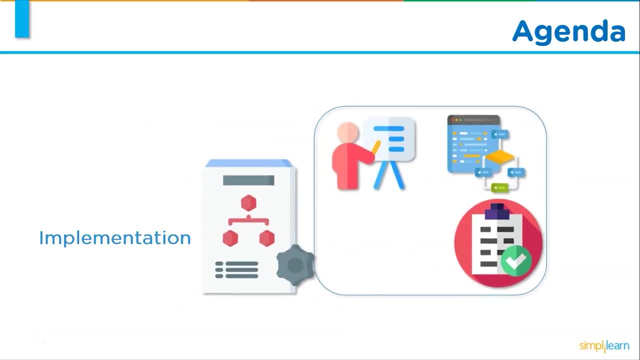 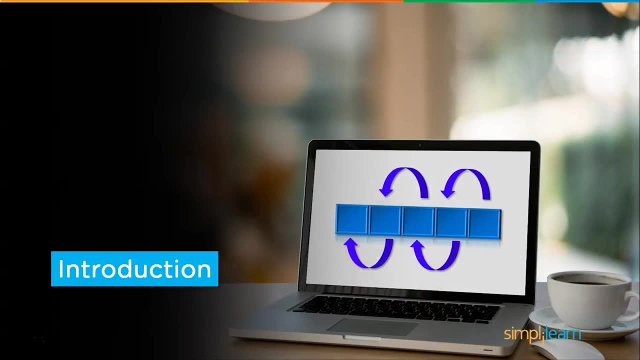 Algorithm. After that, we will implement Radix Sort Algorithm in the code editor. Finally, we will sum up what we have learned from this session. But before we begin, make sure you have subscribed to our YouTube channel and clicked on the bell icon below, so you never miss an update from Simply Learn's YouTube channel. 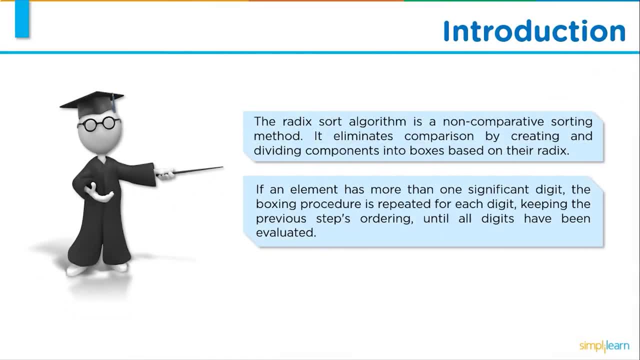 So, without any further ado, let's get started with an introduction to Radix Sort. Radix Sort is a non-comparative sorting algorithm. It avoids comparison by creating and distributing elements into buckets according to their radix, And for elements with more than one significant digit, this bucketing process is repeated. 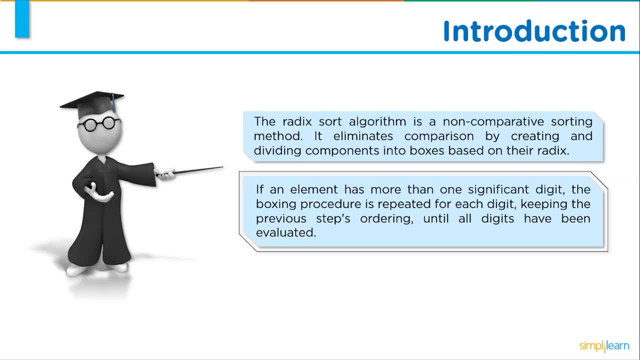 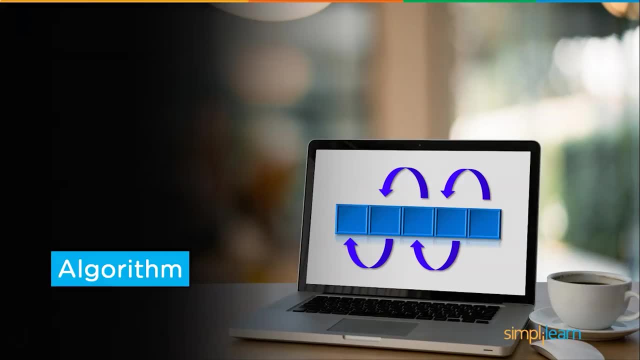 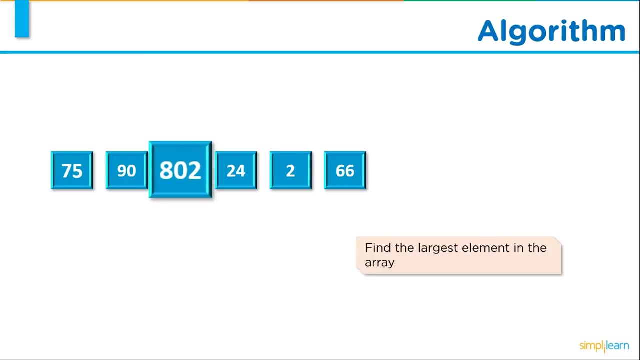 for each digit, while preserving the ordering of the prior step until all digits have been considered. Now let's discuss Radix Sort Algorithm. Let's say we have an array. First we will find the largest element in the array to decide maximum number of significant digits. we will need to compare to sort this array. We will 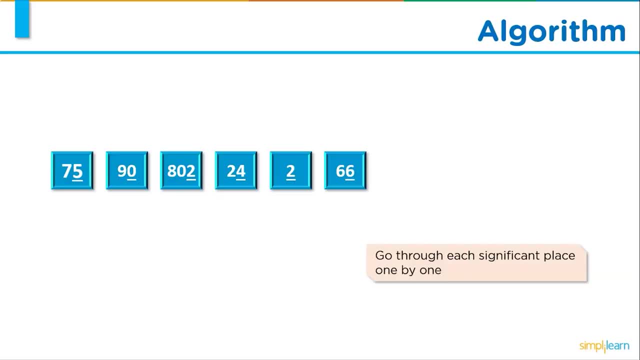 go through each significant place and sort the array one by one. First we will sort the array according to the units place, then we will sort according to tenth place, and then we will sort according to hundreds place, and so on till the array is sorted. 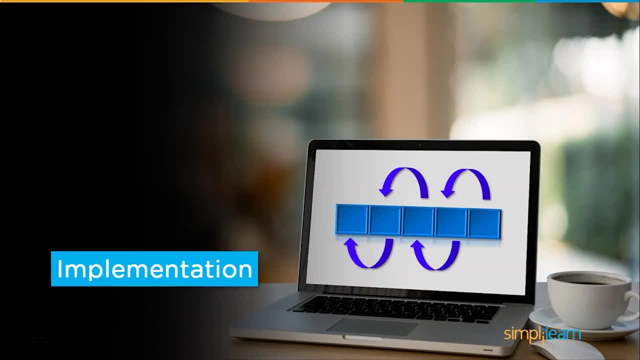 We have now introduced the Radix Sort algorithm. Let's implement this algorithm in the code editor. We will start with the Utility function to get the maximum values in this exists array. If the parameter r is equal to the by the limit of t, then we will add a functionNice. 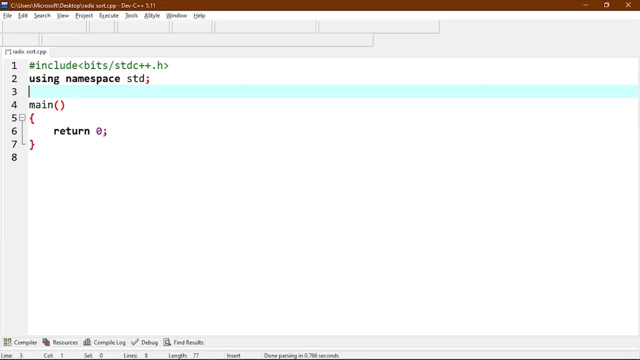 like a string to get the maximum value in the array, So int get max with an argument as array: arr size n. We will declare variable int mx is equal to arr at 0 and we will write a for loop where int i is equal to 1 to i less than n at i++. 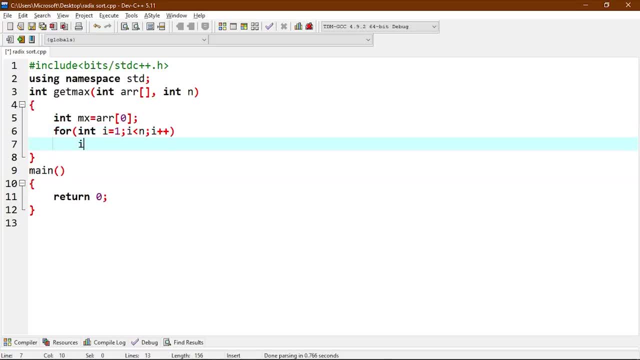 if ARR at i is greater than MX, then MX will be equals to ARR at i, and then we will return the value of MX. Now we will write a function to do counting sort of array, ARR according to the digits represented by exponent. So void, count sort. 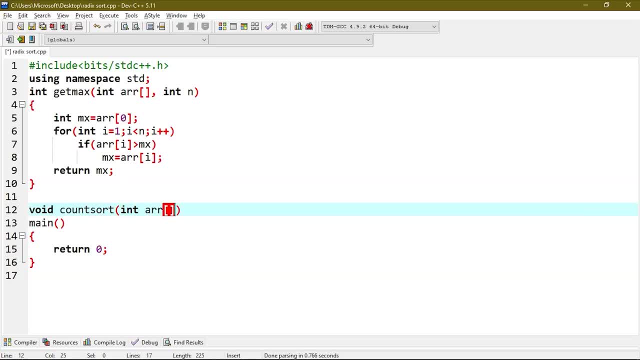 at int ARR, comma int N comma, int EXP. We will declare an integer array output, int i comma account array func of size 10, where all elements are zero. Now we will store the count of all the elements of the array ARR. so for loop per falsetto, i is equal to zero of i less than N. 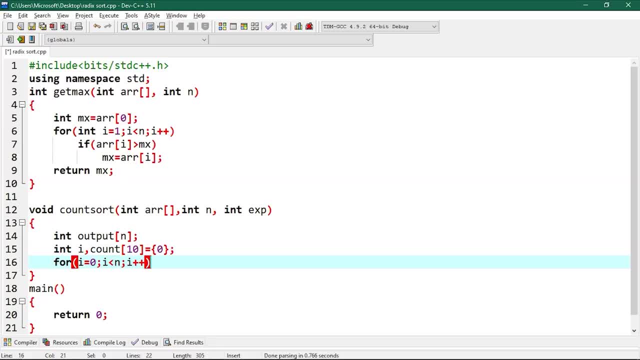 to I plus plus count. error at I divided by exp modulus of 10 plus plus. now we will change count I so that count I now contain actual position of this digit in output. so for I is equals to 1 I less than 10, I plus plus. 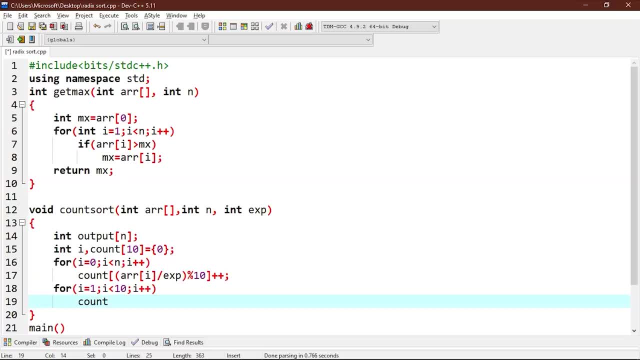 count I plus equals to count I minus 1. Now we will build the output array. so for loop at I is equals to N minus 1 to I greater than equals to 0. so for loop at I is equals to N minus 1 to I, greater than equals to 0. 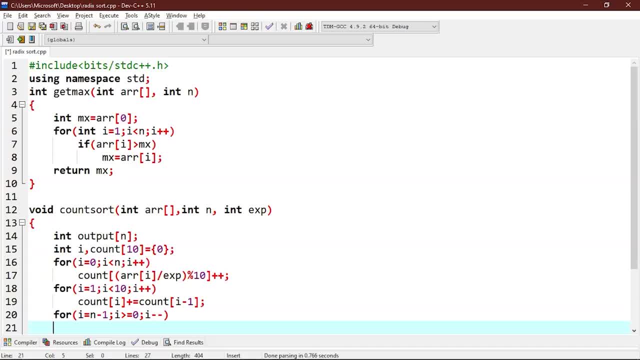 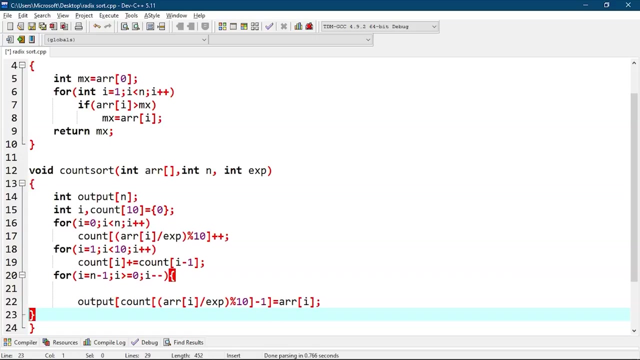 and I minus minus output. count ARR at I divided by EXP modulus 10 minus I minus minus output. ARR at I divided by EXP modulus 10 minus 1 is equals to ARR at I. and now count: count ARR at I divided by EXP modular 10. 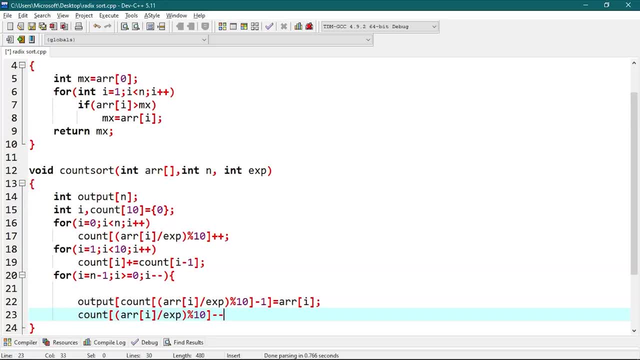 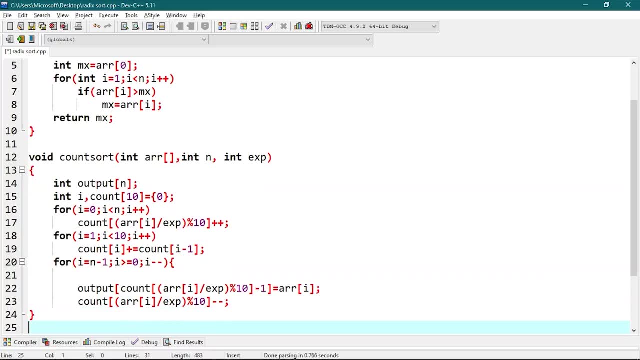 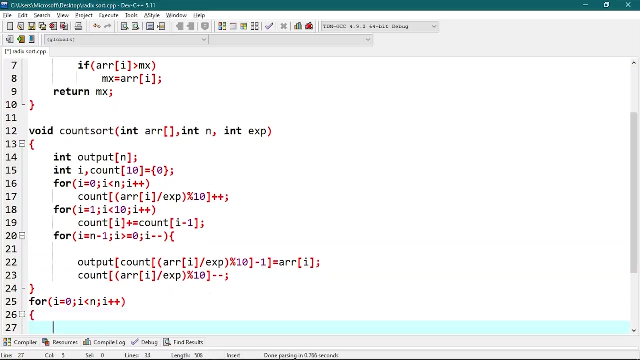 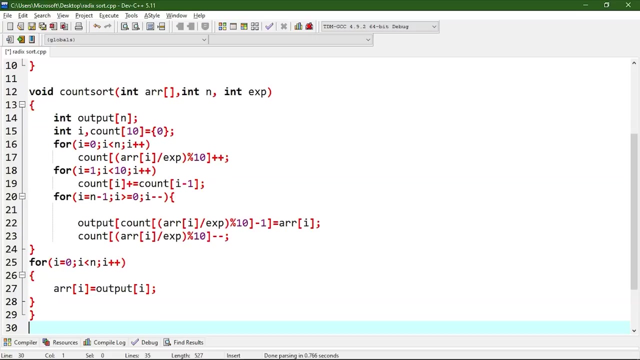 minus minus. now we will copy the output array of ARR so that ARR now contains sorted numbers according to the current digit. so for I is equals to 0. I less than N, I plus plus ARR. ARR at I is equals to output at I. now let's write the mean function that will sort the ARR using radix sort. 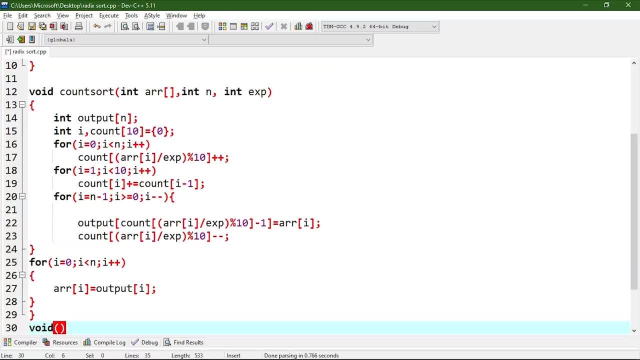 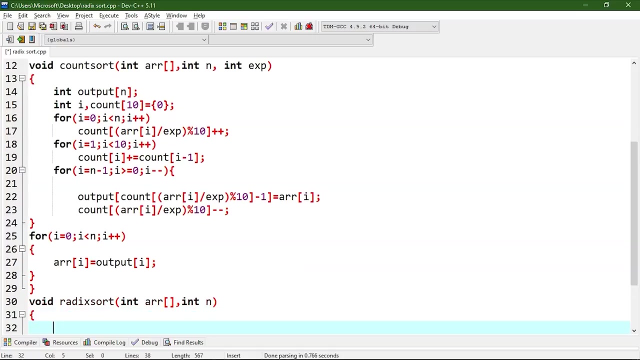 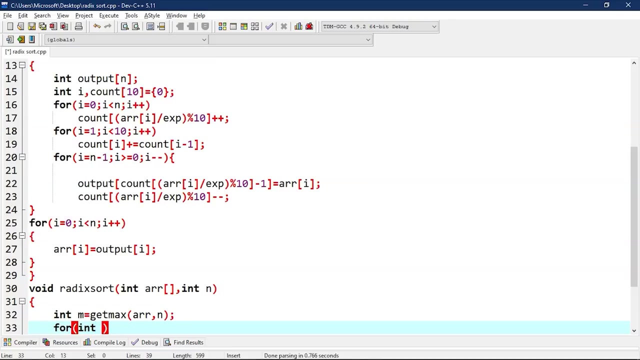 so void radix sort: int ARR comma int N. int M is equals to getmax ARR comma N, getmax ARR comma N. in the input result. getmax ARR finish and getmax ARR Enter hard let's call it for. exp is equals to 1 and m divided by exp is greater than 0, while exp multiplied 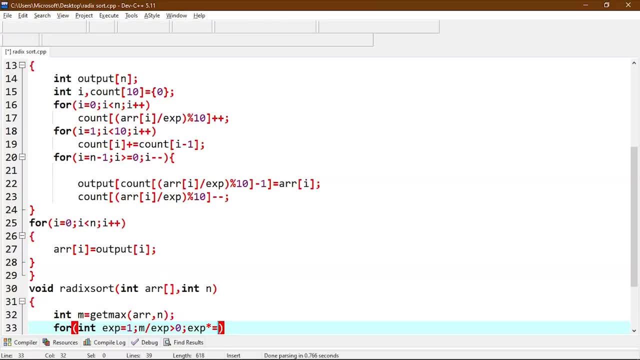 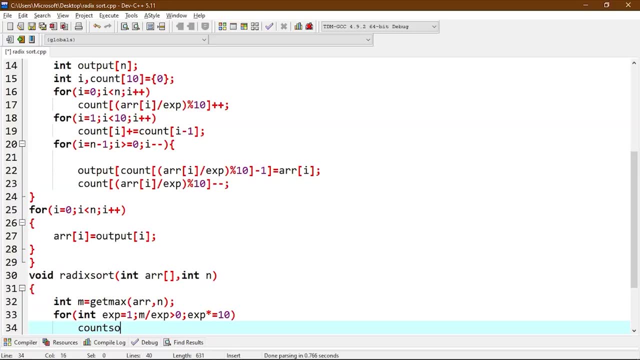 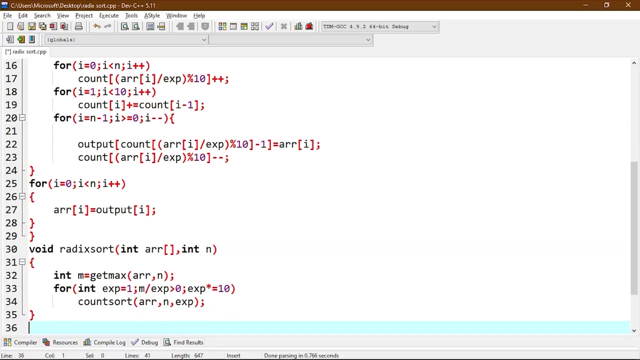 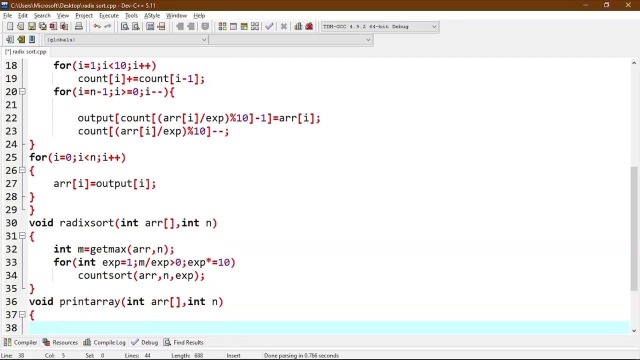 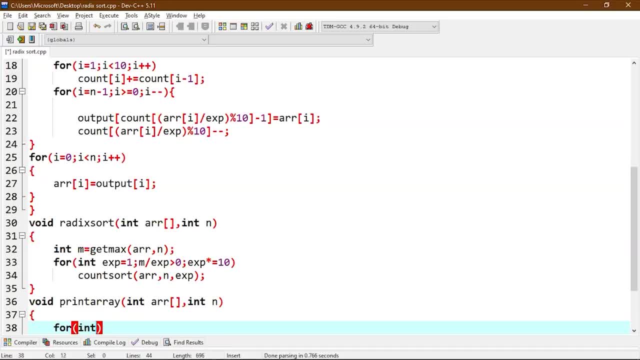 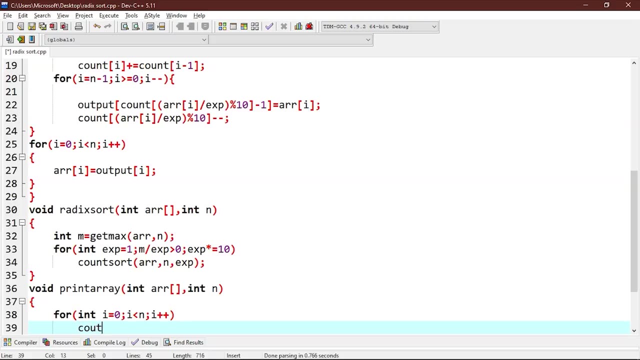 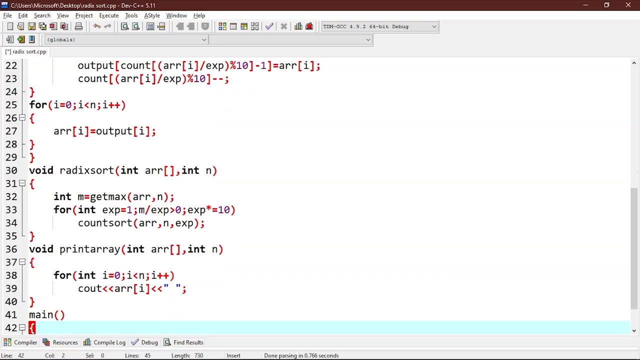 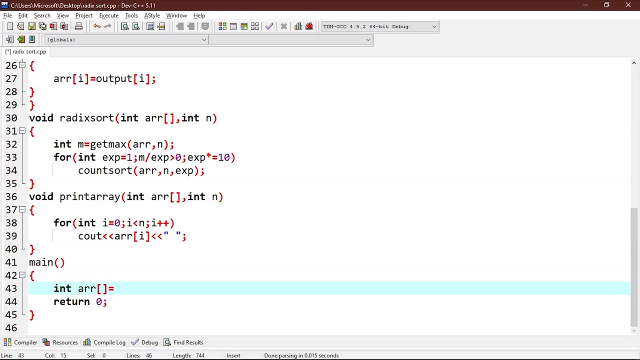 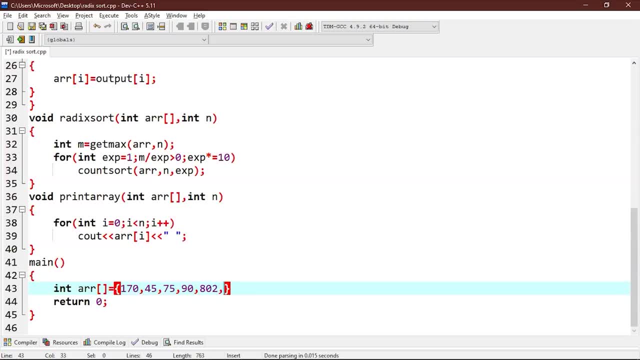